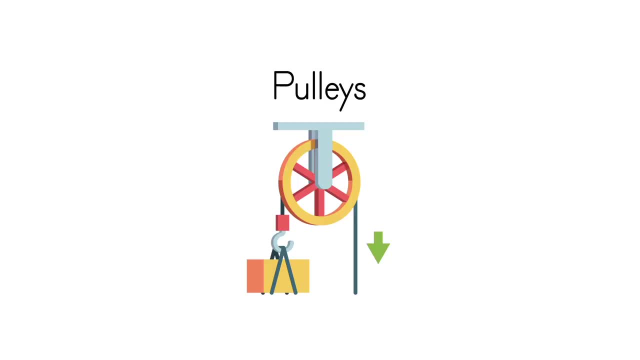 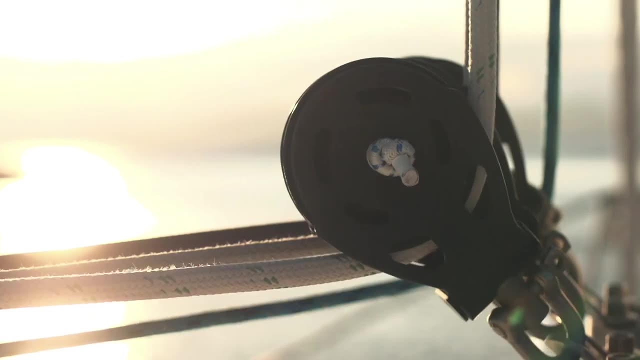 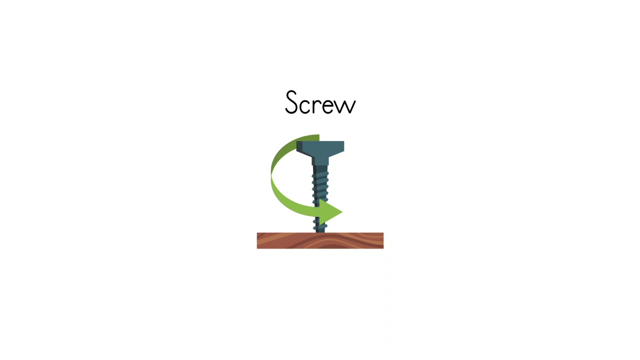 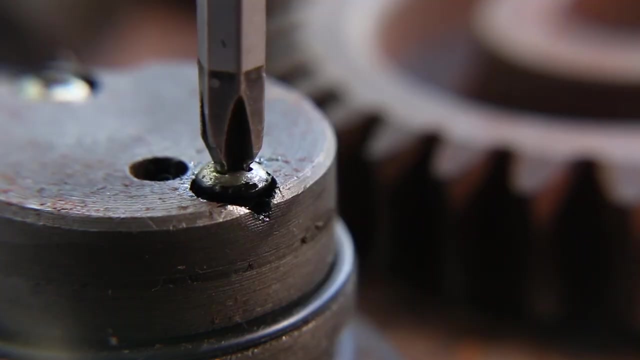 the wheel that carries a chain, rope or belt around its rim can be used to lift heavier weights than a person can lift on his or her own. last but not least is the common screw. the ridges running around the body of the screw allow us to use screws for tightening, fastening or lifting objects you may think of. 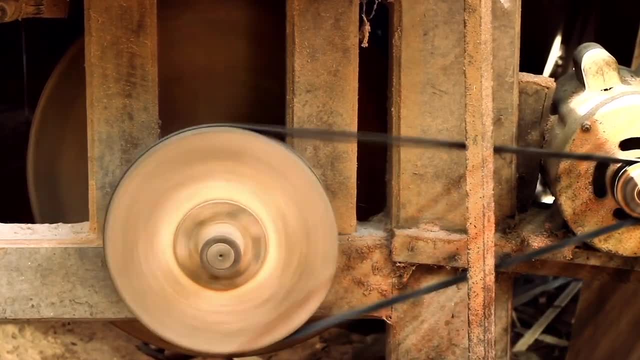 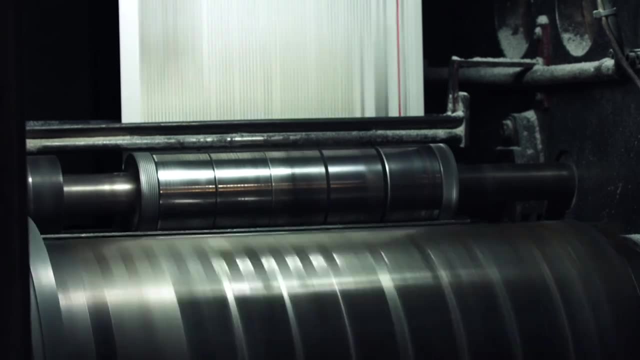 machines as modern inventions, but there are a lot of other ways we can use the modern inventions, but they have actually been around for a very long time, making work easier and more complex projects possible. That is their main purpose – machines are created to help us accomplish work. 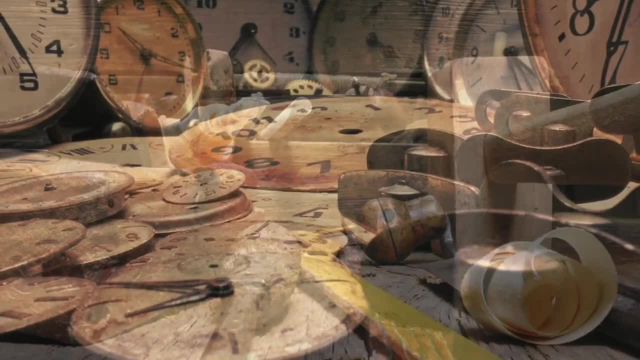 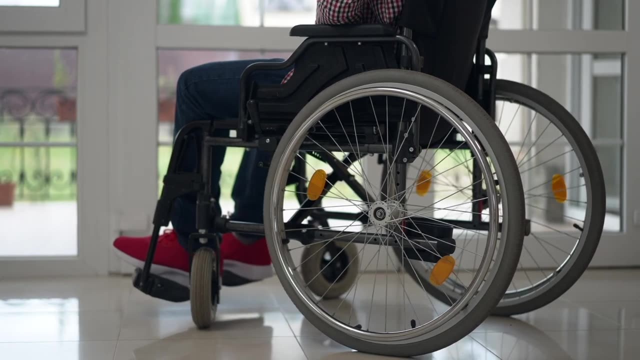 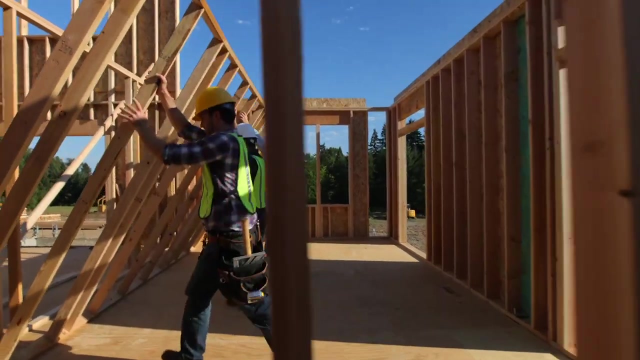 You may think that these inventions are too common sense and uncomplicated to have made much difference in people's lives. but consider the way our lives would be different without the wheel or the screw. Could we be able to build houses as easily and sturdily without metal screws to hold? 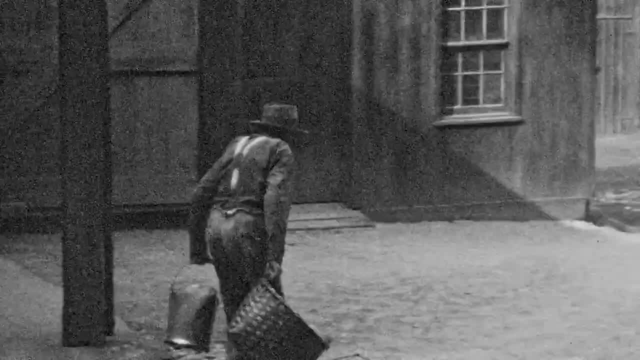 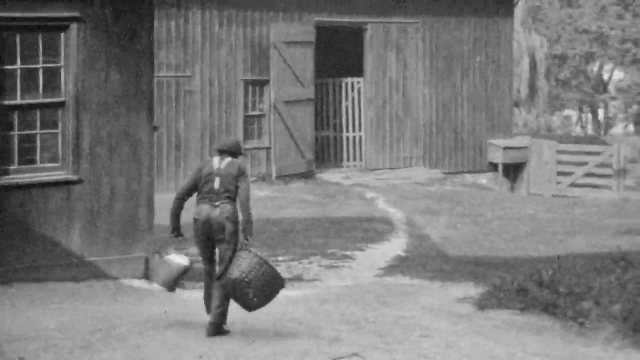 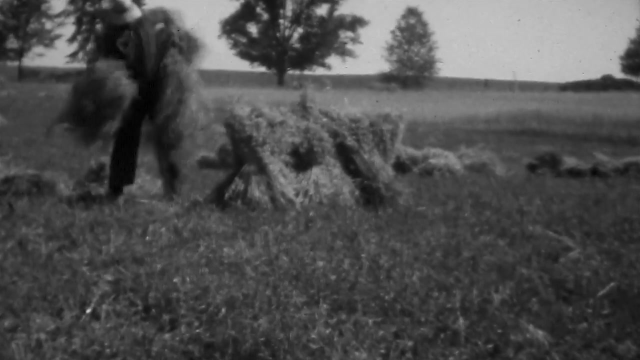 the wood together. As another example, imagine a farmer long ago trying to transport his harvest to market. One way he could get his harvest there is by carrying it himself. But one person can only carry so much weight and it would take the farmer a lot of trips. 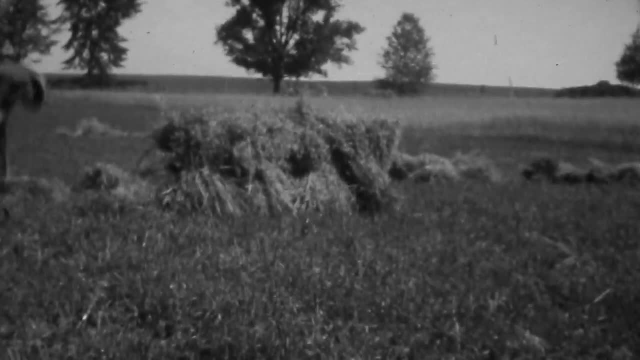 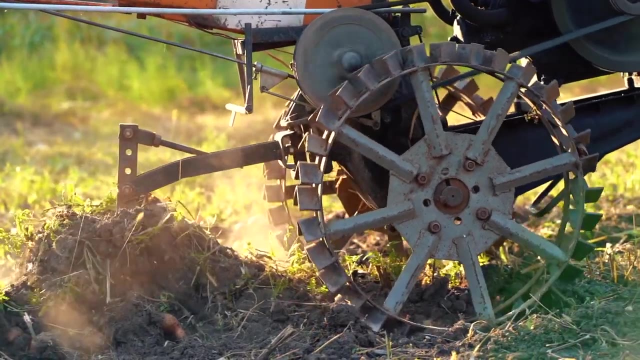 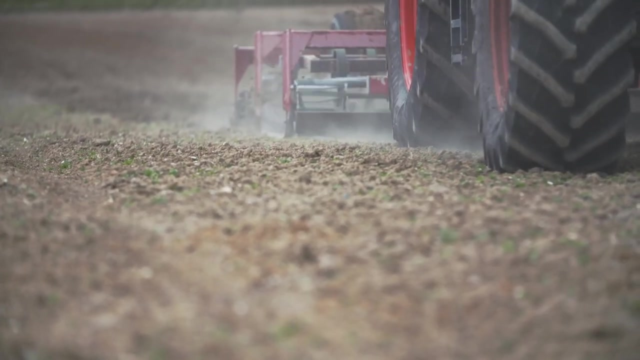 and effort to move all of his crops by hand. The invention of the wheel, One of the most important simple machines of all time, revolutionized the way humans moved objects and transported themselves around. This simple, life-changing machine allowed and still allows the farmer to accomplish. 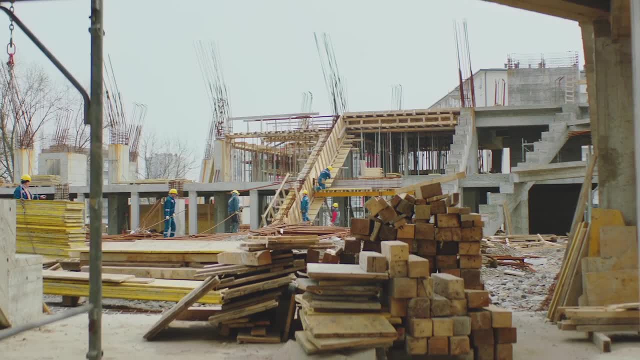 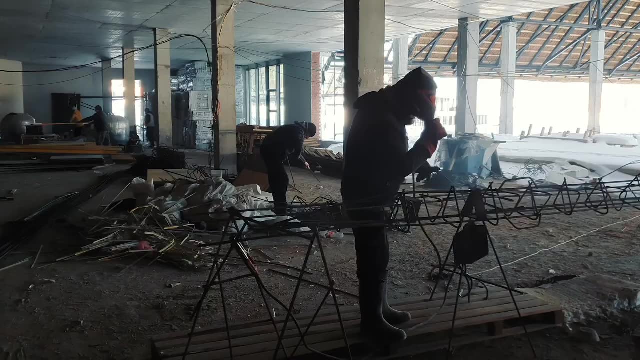 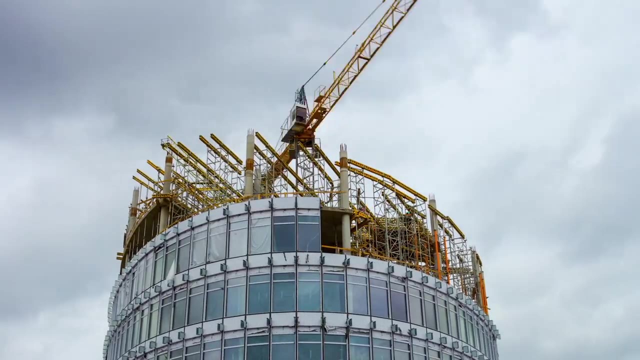 more work with less effort. One area where simple machines have made a big difference is in construction. People have been constructing buildings such as churches, tombs, mansions, mansions and homes and palaces for thousands of years, but over time humans have designed many machines. 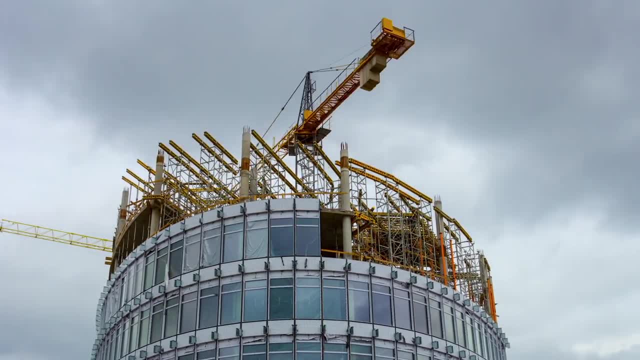 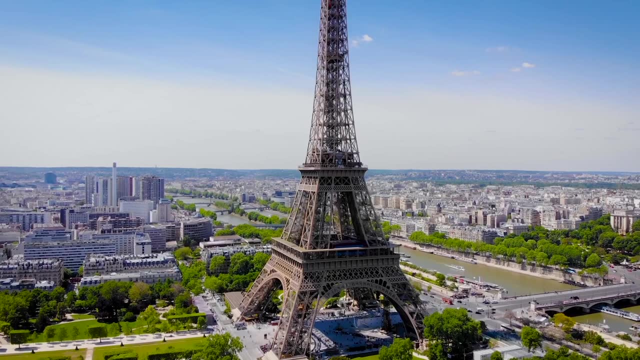 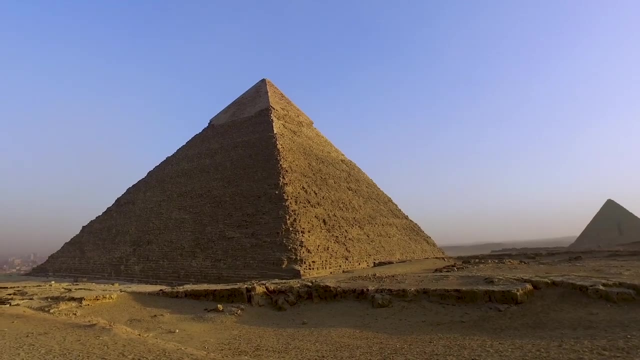 to make the construction of these buildings easier and safer. Can you imagine trying to build the Eiffel Tower in France, over 1,000 feet tall, with nothing but your hands? It would be impossible. Or consider the Egyptian pyramids: These massive structures couldn't have been made without the use of tools and skills.